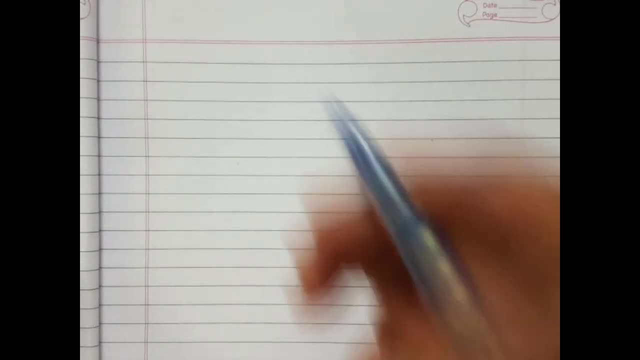 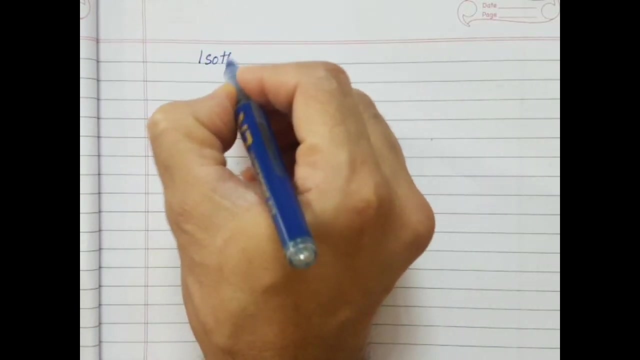 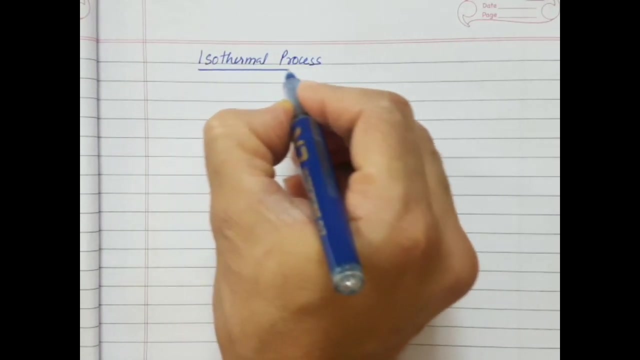 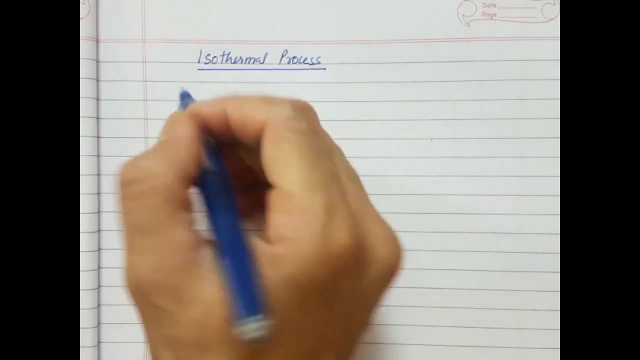 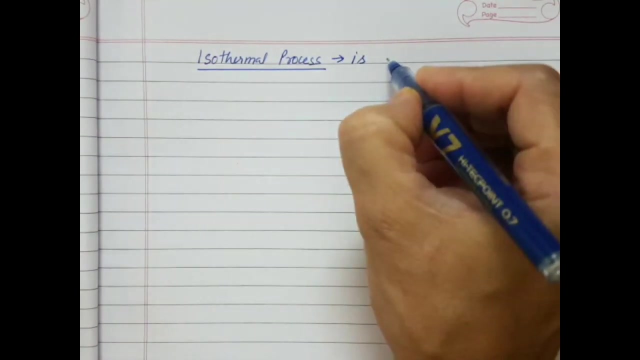 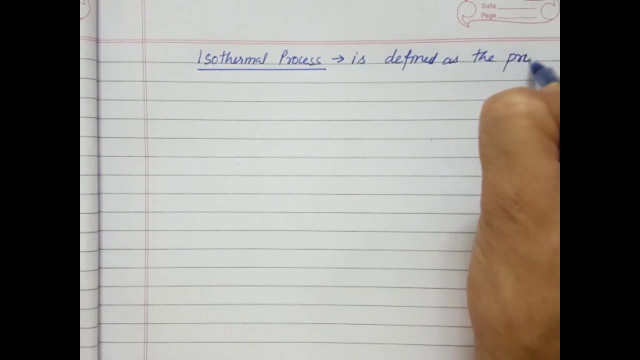 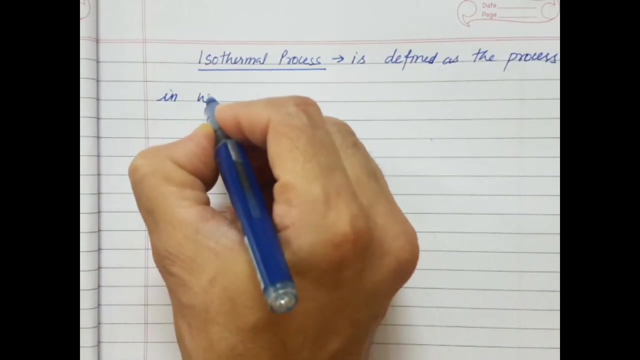 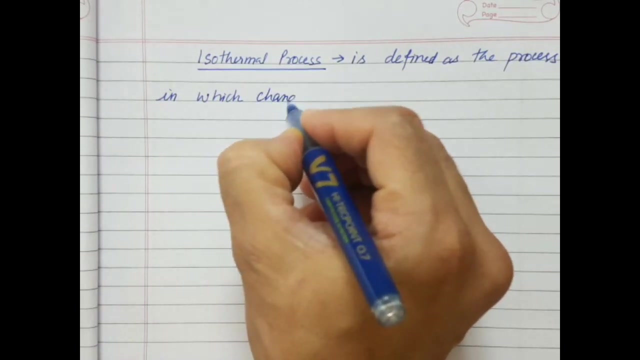 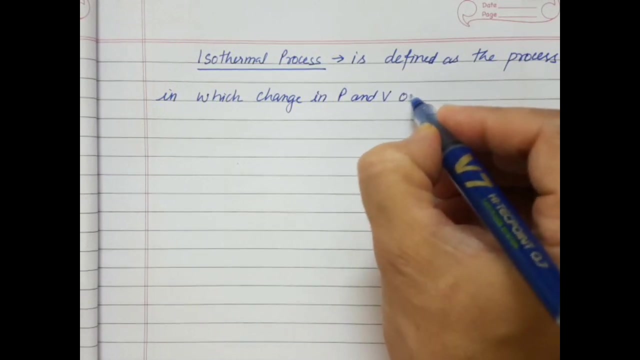 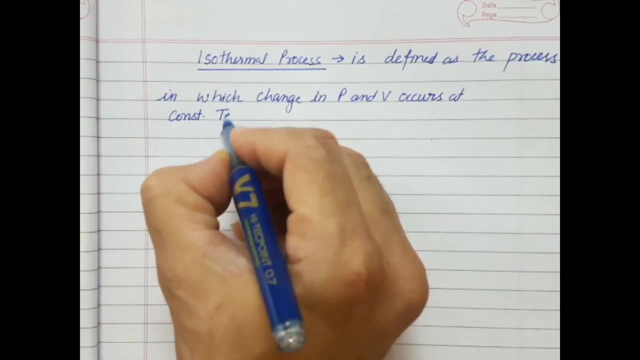 Next we will discuss isothermal process Now, as, per definition, the isothermal process may be defined as. let us write down the definition: it is defined as the process in which change in pressure and volume occurs at constant temperature. So what does it mean that during this process, 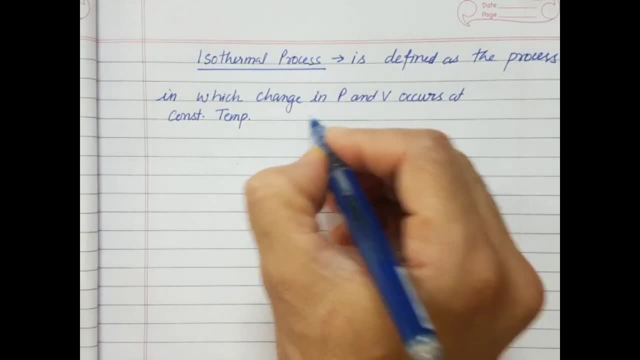 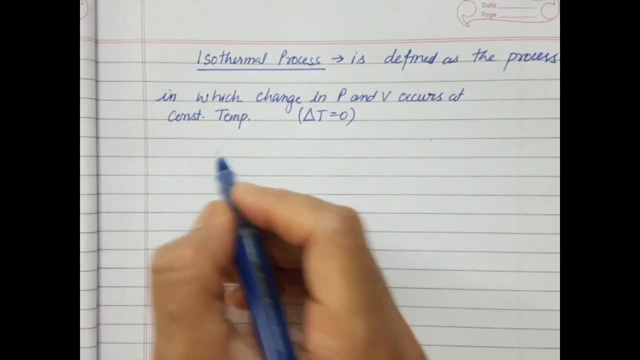 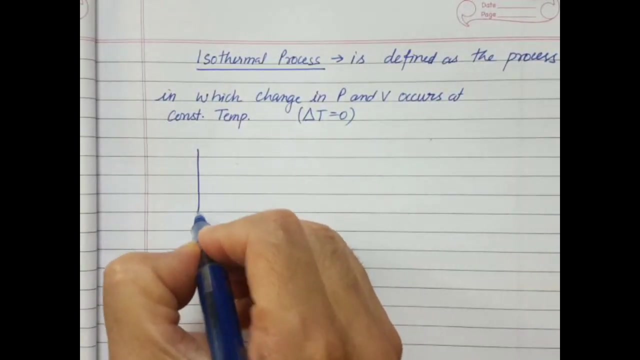 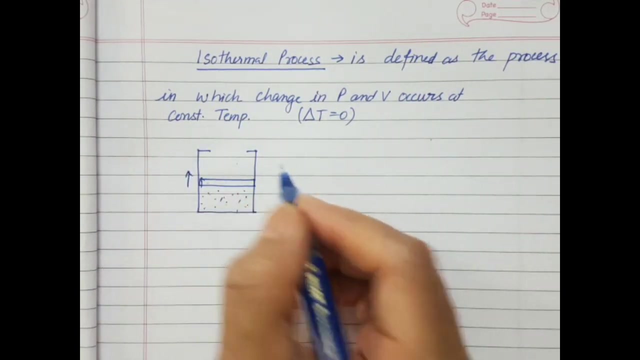 the temperature remains constant, So delta T is equal to 0 throughout the process. So let us try to understand the process in a. Now let us take a look at the piston cylinder arrangement. In the zoom there is a gas which is kept inside the piston and the cylinder. Now this is. 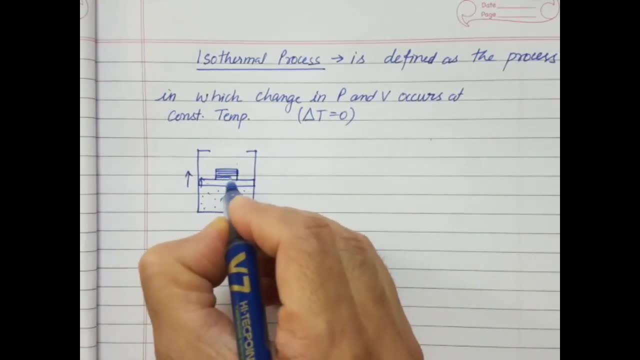 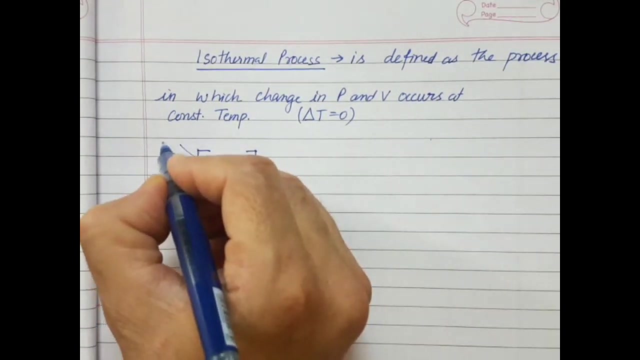 the gas. Now this piston is free to move. Now let us assume we have put the weight. Sir Piston is 1933.. Sir, which is in very, very small strips, in the form of small steps and the initial coordinates, let us say, has p1, v1 and t1. now let us do: I remove a very small way. 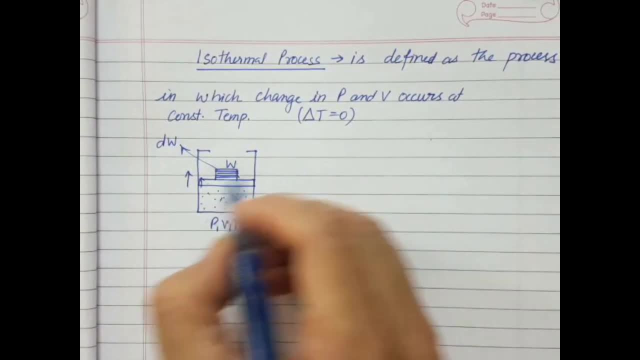 DW, I remove this weight. so what will happen when I remove the very you can says fraction of weight from this piston, the there was, there will be a very, you can say slightly change in pressure acting on the gas. so this piston, in order to- and this you can say- equalize the process, this piston will move in. 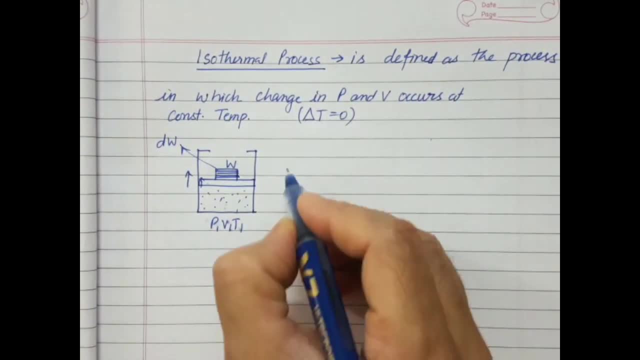 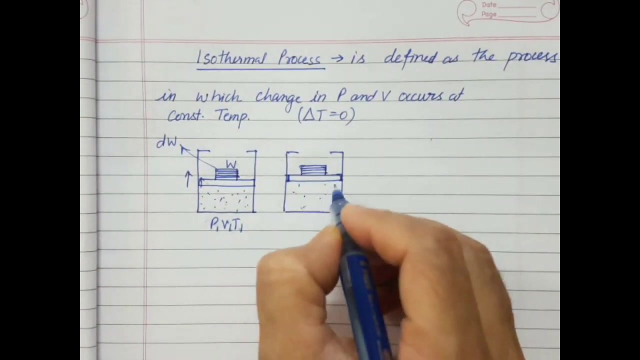 backward direction, in upward direction. so it will go into the new position just to good. take the system in equilibrium conditions this time. move slightly over that option. now this is the new one. units pressure, because P 2-1 become sweet doing temperature. we can see 2. 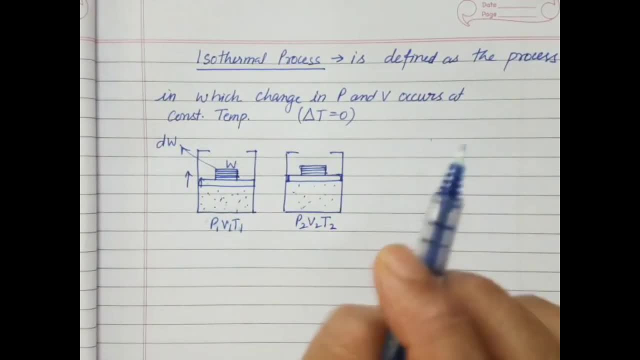 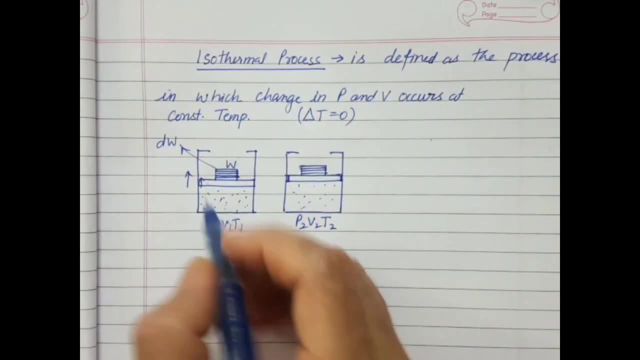 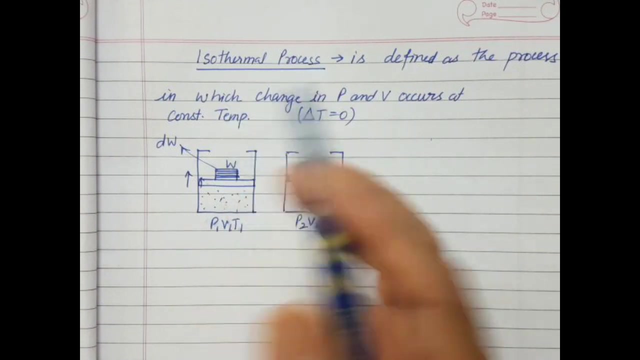 now the. and you must keep in mind that during ice, with her first process, the walls of the system should be very conductive, because when I remove the weight, this should not be any increase in the temperature. So in order to keep the temperature constant, when I remove the weight some, the pressure is, you can say, reduced and the temperature of the gas may be reduced by some amount. So in order to compensate for the temperature, that heat may come inside the system so that the temperature remains constant. 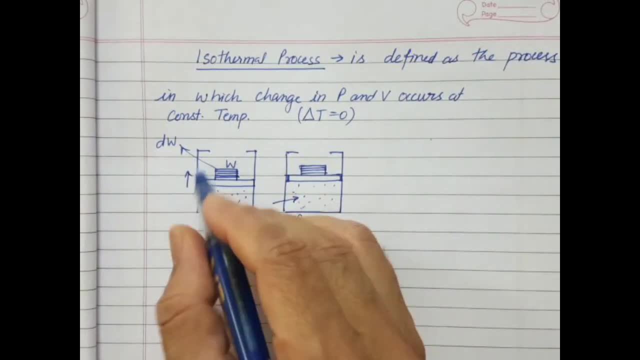 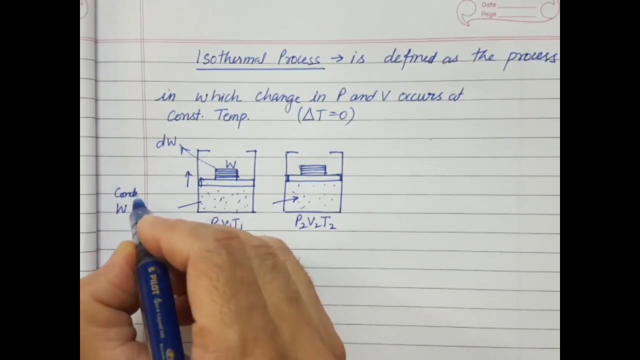 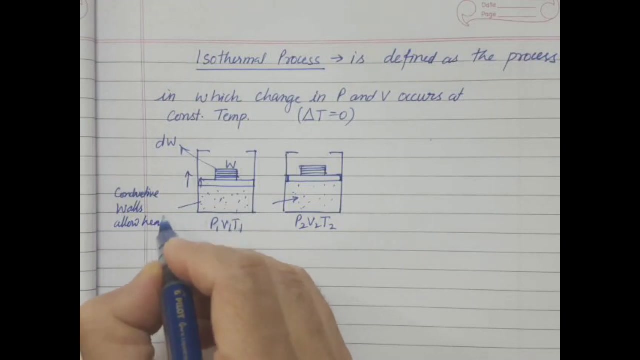 So for this, the walls should be very conductive, So you can write here: conductive walls. Walls Allow heat transfer, So this is a… Apart from this… Apart from this, there are many more things which we need to know about isothermal process, like this process should be carried out very, very slowly. 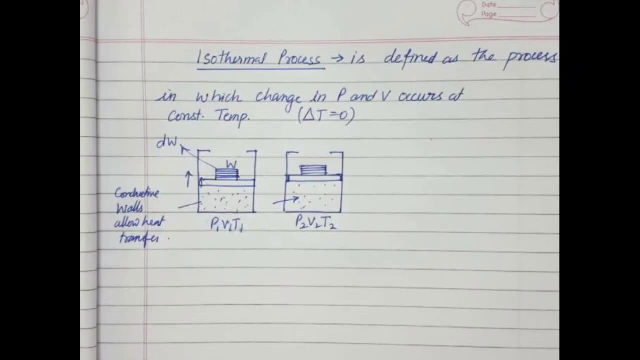 Now, what is the reason behind it? Why it should be carried out very slowly? Because, as we know that during this process, we need to keep the temperature constant. Now imagine any type of process occurs like we have removed the weight and in doing… While doing so…. 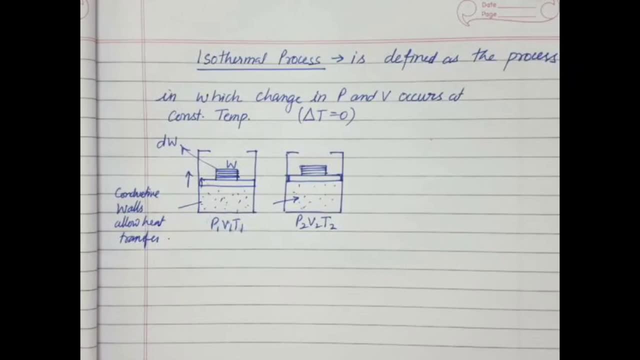 The system will move backwards and pressure will reduce. So in this process the temperature may lower, but we need to keep the temperature constant. So the heat must be supplied during this process. So the process should be carried out very, very slowly so that during each step the temperature remains constant. 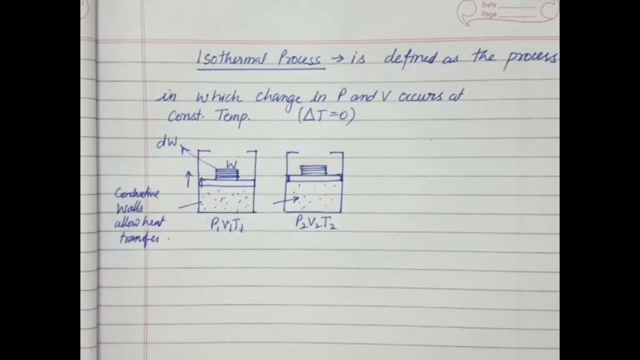 So you can easily correlate this process with the quasi-static process. It is just like a quasi-static process, in which it should be carried out in a very, very small steps, And so it should be… It need to be undergo in a very slow manner. 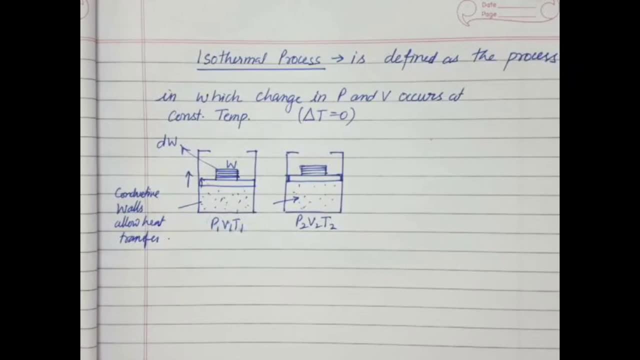 Now example of this isothermal process in daily life is like we design our air compressors based on isothermal process, because isothermal process corresponds to the lowest amount of work. Apart from all the processes, Isothermal process needs lowest amount of work input. 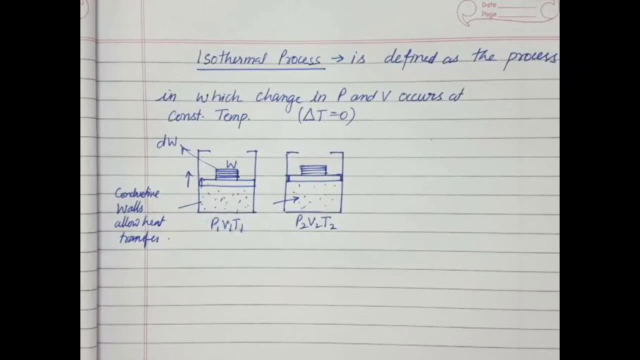 So air compressors are usually designed with the very slow speed motors. Slow speed motors So that during the air compression process the heat generated during the compression work should be dissipated out of the compressor walls. So as more slow will be the process, more will be the work…. 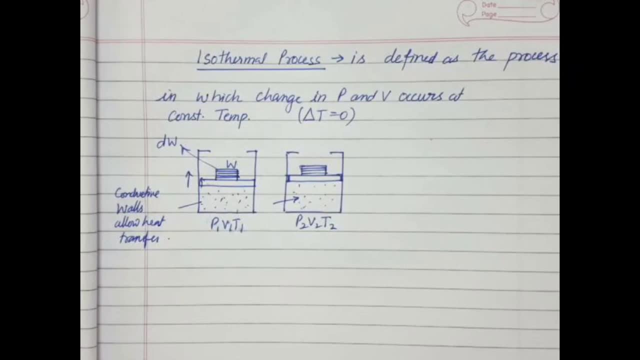 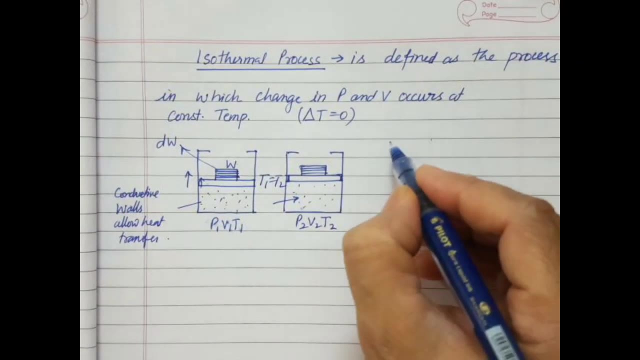 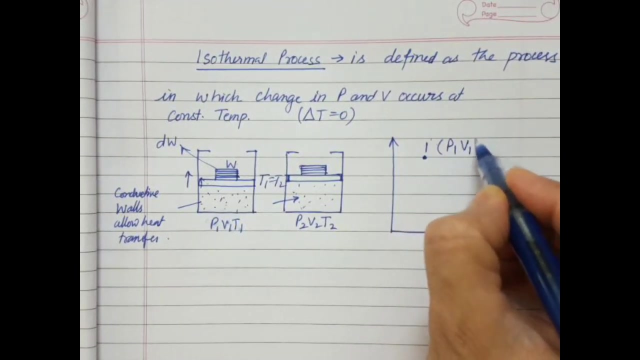 More will be the efficiency of the compressor and necessary amount of the work will be required to be transferred. So air compressor is a good example of isothermal process. Let us draw this process on pressure and volume graph. Now let us say this system is at point 1, with coordinates P1 and V1.. 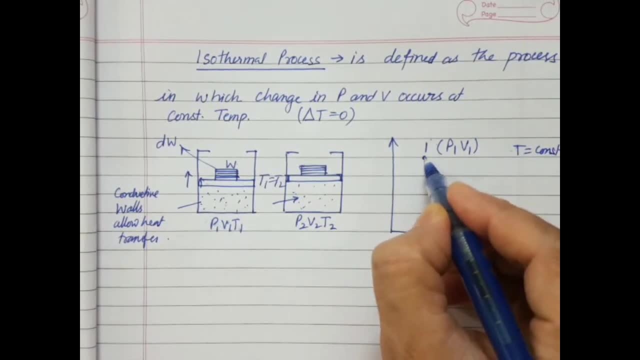 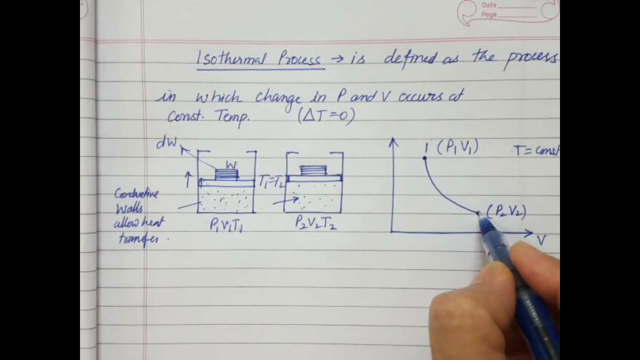 Temperature is equal to constant And it undergoes a process like this and takes a new coordinates: P2 and V2.. So, like this, like this: Here is V1.. Here is V2.. Here is P1.. Sorry, P1. 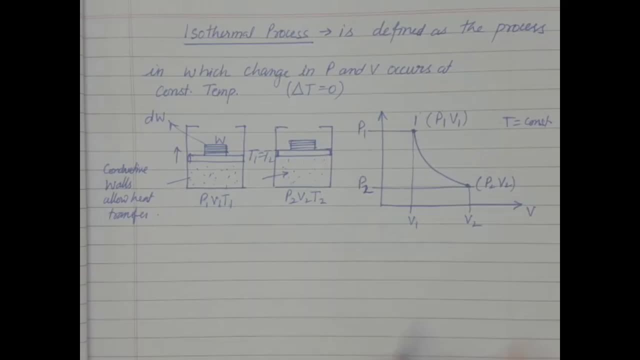 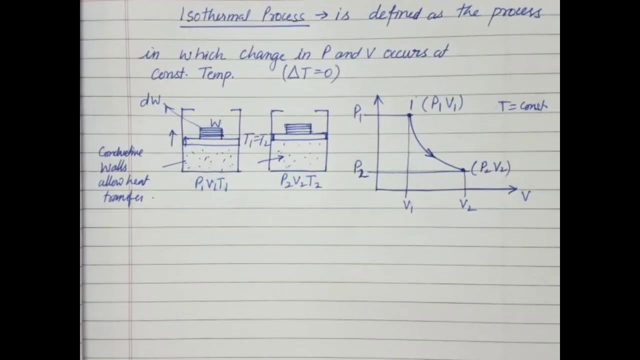 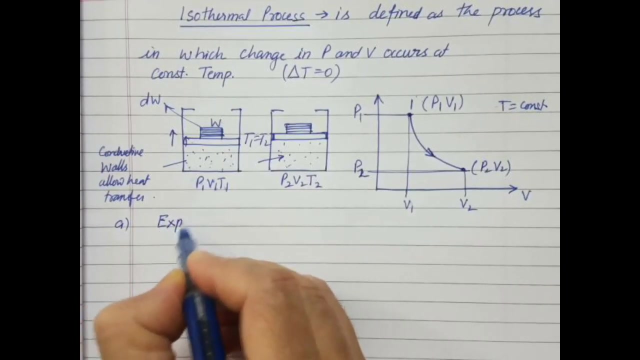 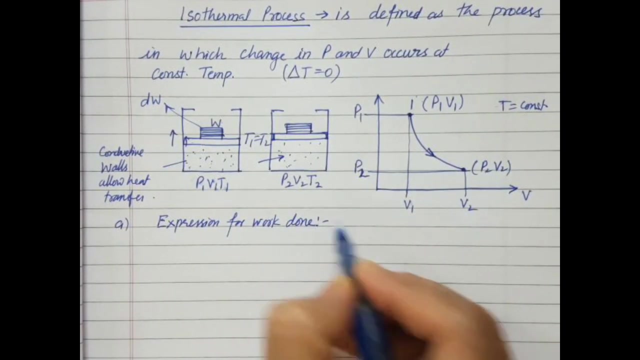 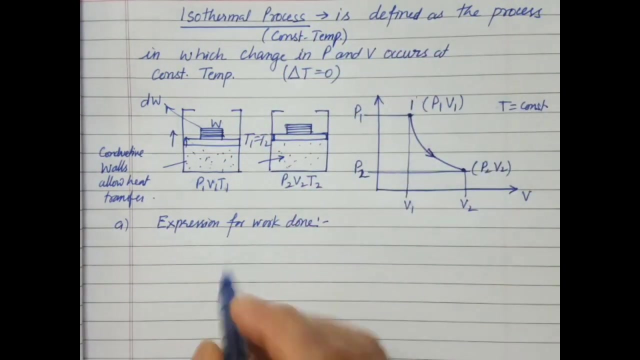 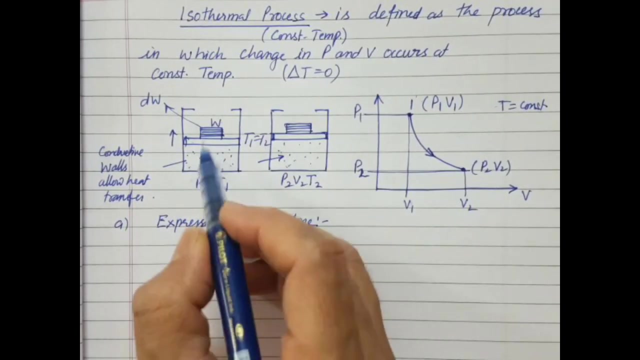 Here is P2.. So this is your process. Now let us calculate the work done: Equation expression for work done. Expression for work done in isothermal process, Constant temperature. Now, as we remove the very small amount of work, This amount of, you can say weight from the piston. 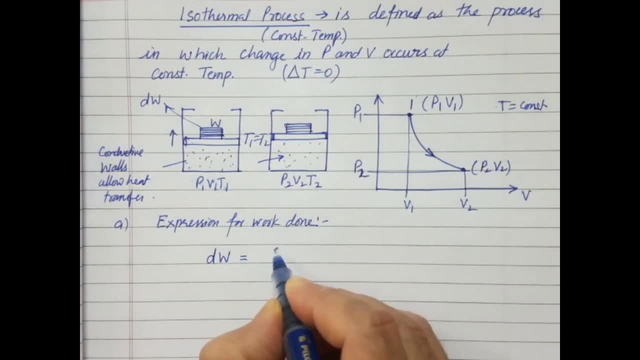 So very small amount of work can be calculated by integrating the pressure and volume between 1 to 2 states. So work done is equal to P times V2 minus V1.. Now here you know that P into V is equal to constant according to Boyle's law. 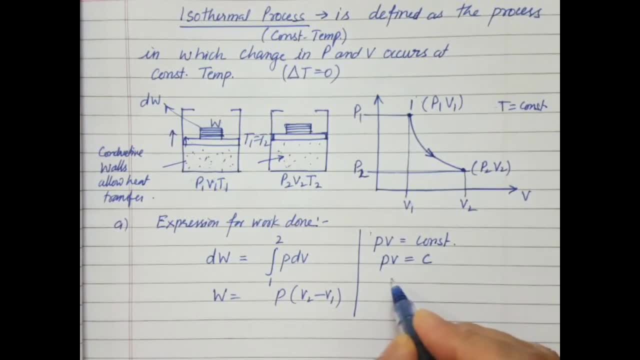 And we can write: as: PV is equal to C, And we can write: P is equal to C by V. Now here, just replace the pressure value of pressure with C and V, So it becomes C by V, V2 minus V1.. So we can also write in terms of log: 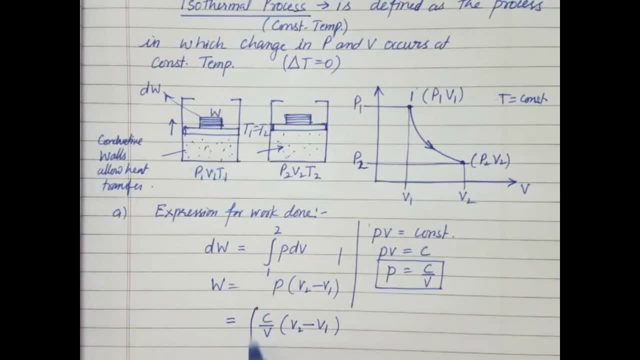 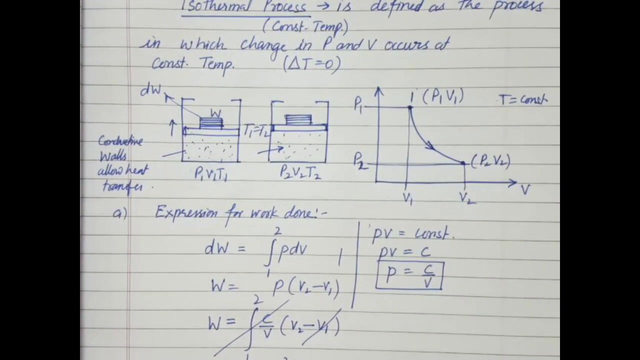 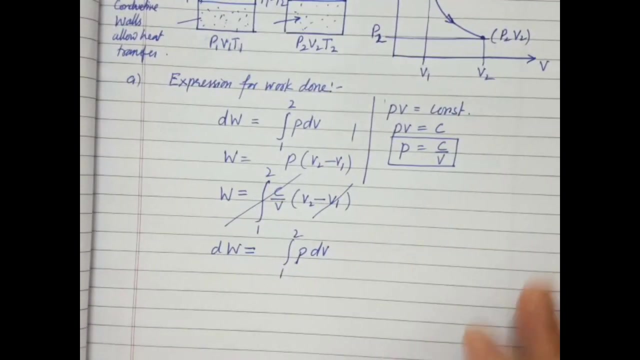 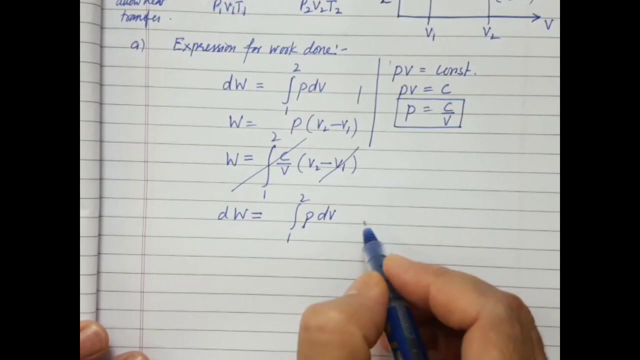 Natural log. If we integrate this here, So W2.. So W2 between 1 and 2. Let us say DW is equal to 1 to 2. P into DV, So this is equal to Just hold on. 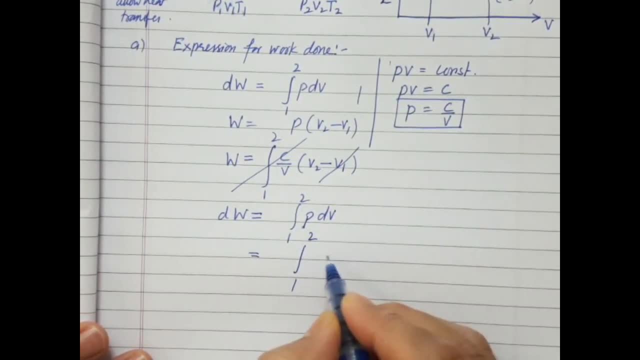 Now we can replace the value of 1 to 2.. C by V into DV, So this becomes C into log of V2 by V1 log E. Now we can also write it as C times. Now PV is equal to PV is also equal to MRT. 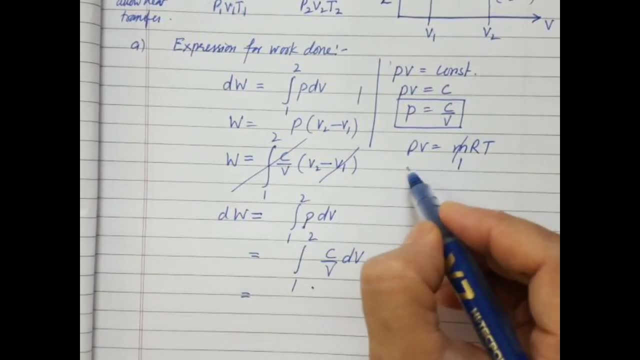 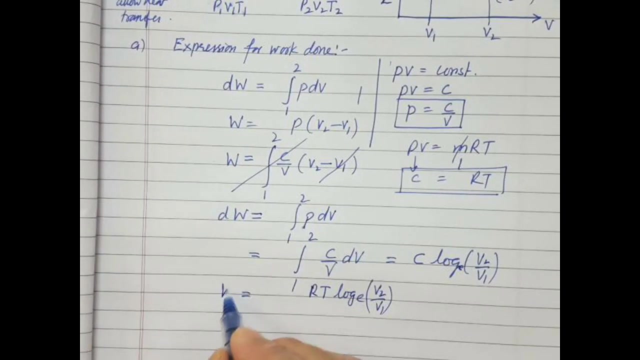 Taking mass is equal to 1.. So PV Or C is equal to RT. From here we can replace this RT log of E into V2 by V1. So we can write it as Work. done is equal to This in case of isothermal process.